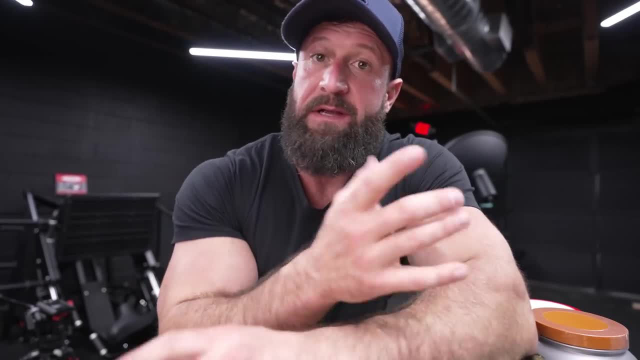 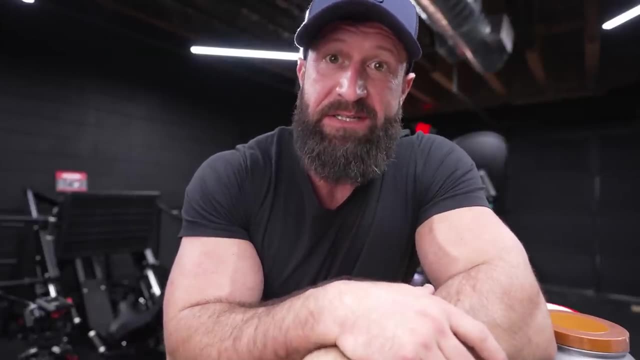 should tell you why. now. the product was great, the company was good. it was none of that. i can only categorize it as cognitive dissonance, which is inconsistent beliefs. my least favorite thing is to go through instagram and see some guy sitting there with whatever product he represents. 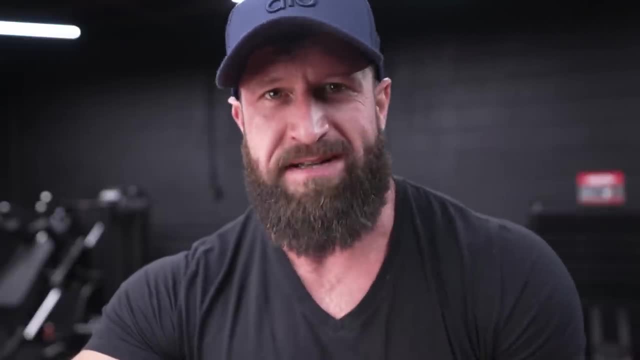 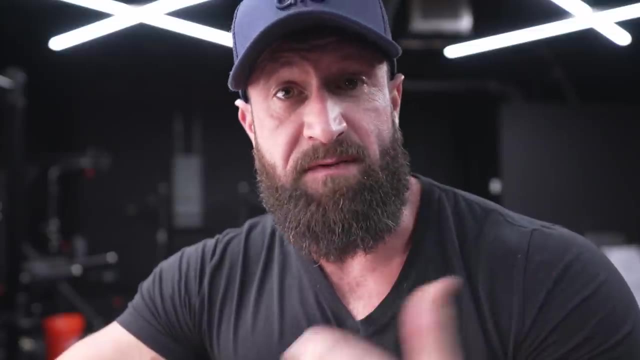 and some sort of caption underneath that says this is the only product i take, because you know that's. that's not how we take supplements. if it's a pre-workout, we find one that makes it feel like the hair on our ears is growing 10 times faster than it should, and 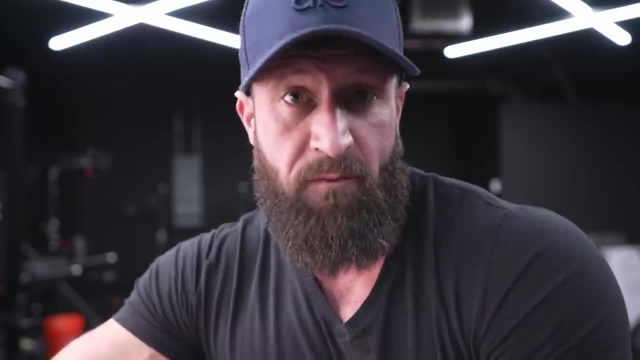 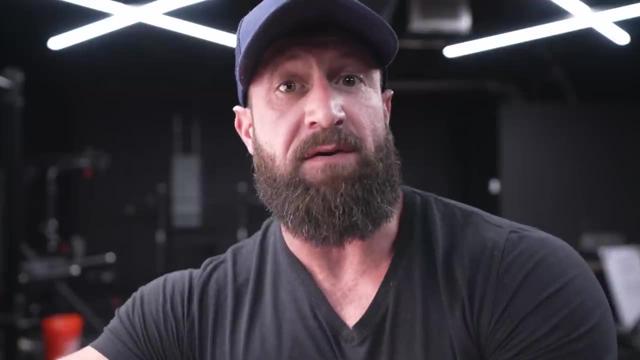 until that starts to wear off, and then we switch to a different brand with a different formula and then we feel that in our plums for a while until that goes away, and then we switch back. protein powders are a little bit different. you find a flavor you like, that you think you can. 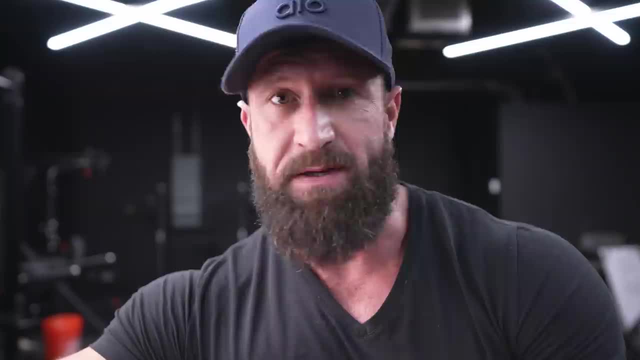 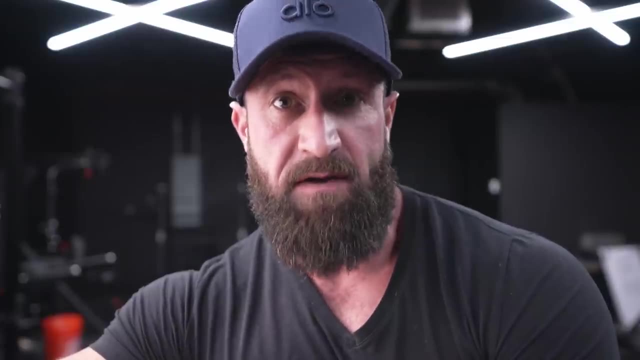 drink forever until one day you want to stop drinking it. and then you want to stop drinking it. wake up, take a sip and throw up in your mouth, because your body's like that's enough. so you go on the hunt for a couple different flavors and you try everything except vanilla, because vanilla 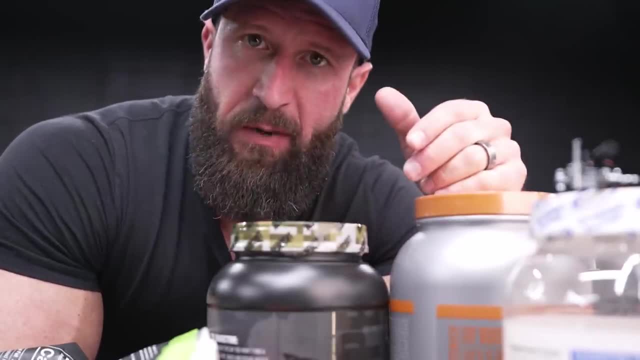 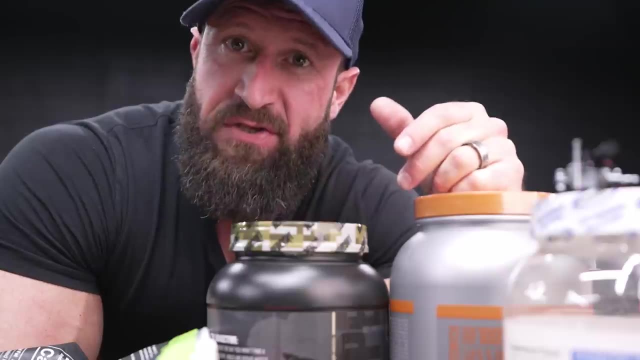 and that's where the cognitive dissonance came from. because i'm not loyal to a brand, i'm loyal to that tingly feeling and if you stop giving it to me, you can off. and if your protein powder starts tasting like because i'm used to it, i'm gonna use a different one, and you should too. 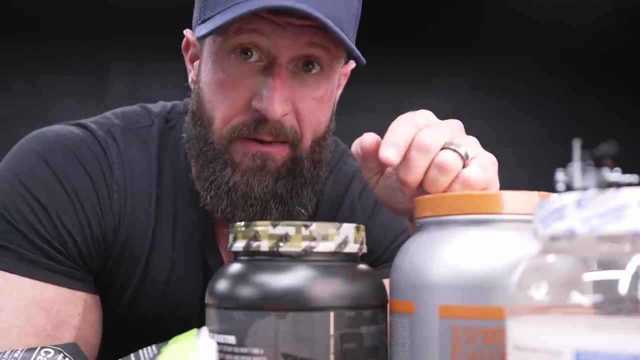 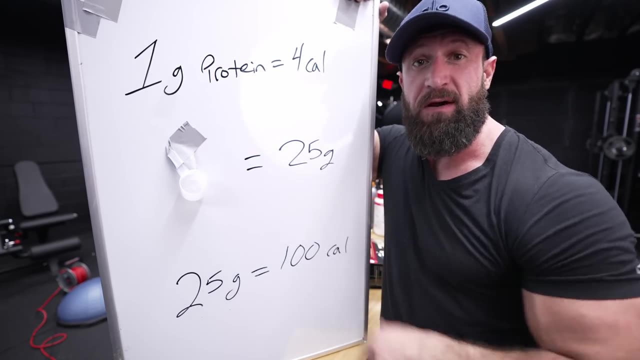 so let's go over exactly what you should look for in your protein powder. all right, let's start with the basics now. one gram of protein is roughly four calories, and most companies try to make their scoop out to be about 25 grams of protein. so that means the cleanest possible scoop of protein should be. 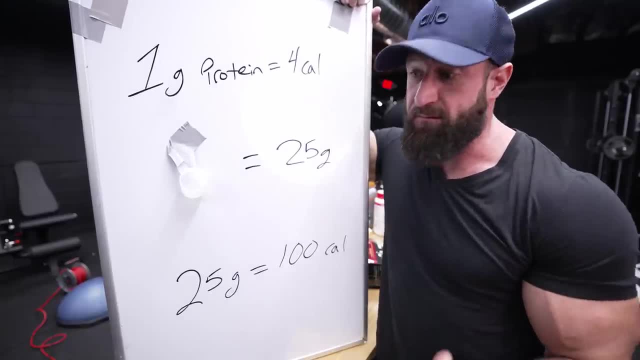 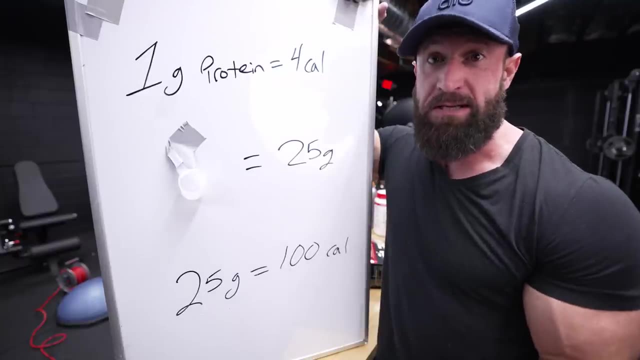 right around 100 calories. but before you run out to your supplement shop and try to find a protein powder that's only 100 calories per scoop, don't do that. that's a rookie mistake. you're gonna end up with an unflavored protein, and unflavored protein is not lacking in flavor. it has one. it's you. 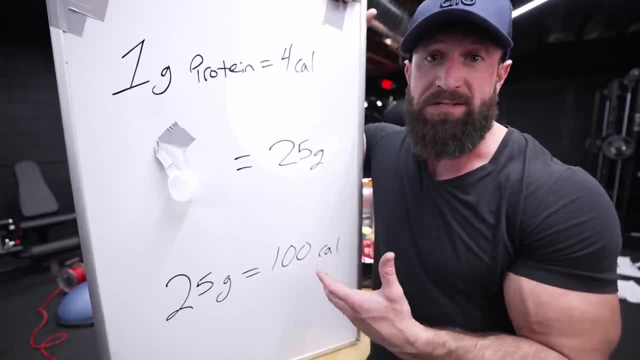 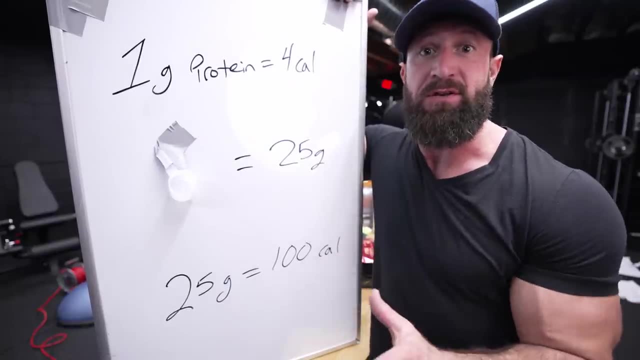 gotta give these companies a little bit of wiggle room to fit in their sweetener profile. otherwise you're gonna have to have that conversation with your wife about why you're not throwing away that unflavored protein that tastes like and you're never gonna drink it. but